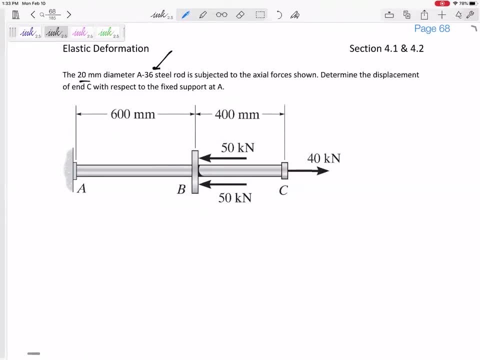 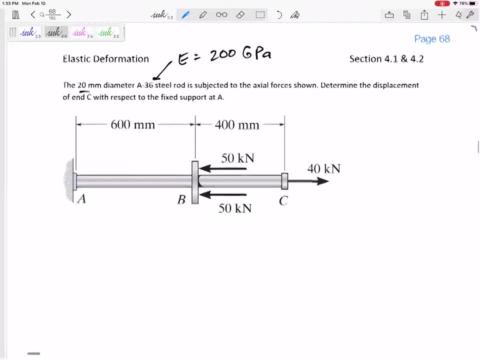 So 20-diameter A36 steel. from the back of the book It's E200GPA. I prefer MPA, but we'll see how our units will cancel out All right. so the E of that material is 200GPA. It's subjected to. 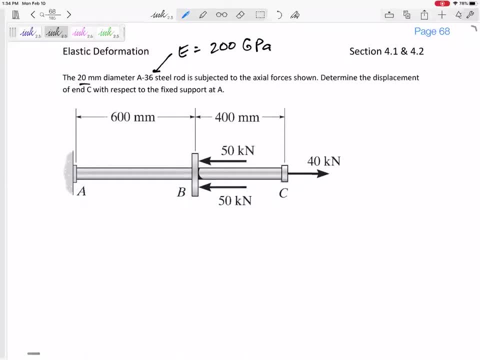 the axial forces to determine the displacement of NC with respect to A. So what's the delta L between A and C? Well, I'm going to break this up and I'm going to find the delta L of that section, the delta L of that section. right, I'm going to sum up these delta Ls. Summation of. 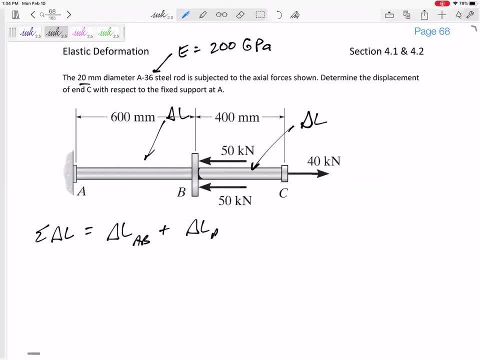 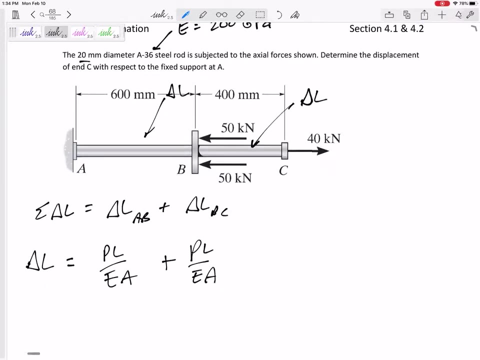 or just say delta L of section AB, delta L of section BC, right? So what is the PL over EA of that section? the PL over EA of that section е are two different p's, you know two different lengths. i think the areas are probably the same. 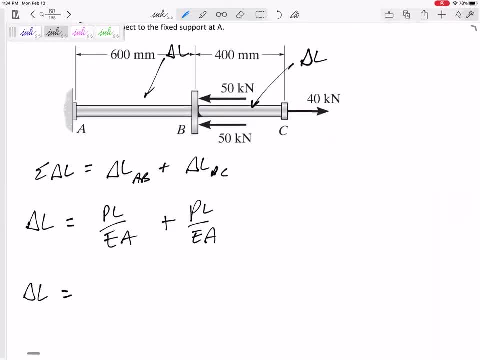 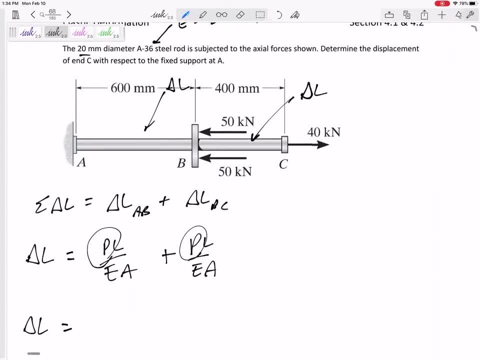 the e's are still the same, all right. so what is the force inside section a b? what is the force inside section b c? i don't know if you are comfortable now to just look at it and see it. let's, let's assume not cut it open and solve for the force inside. so inside section b c. 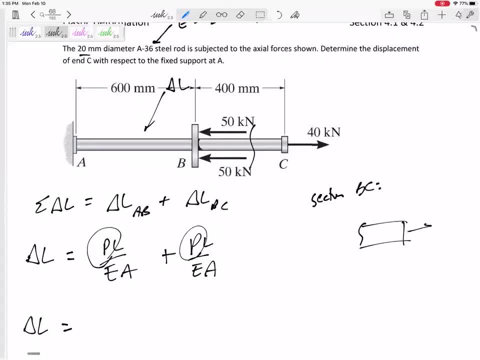 i cut it open. i've got 40 kilonewtons right here. so summing the forces in x equals zero. i would get 40 right. so that force, would it be positive 40 kilonewtons or negative 40? uh, it would be in tension. that would be positive 40 kilonewtons. 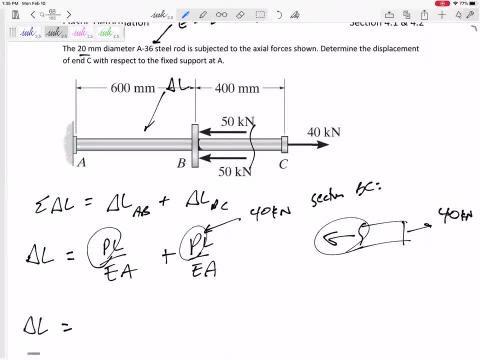 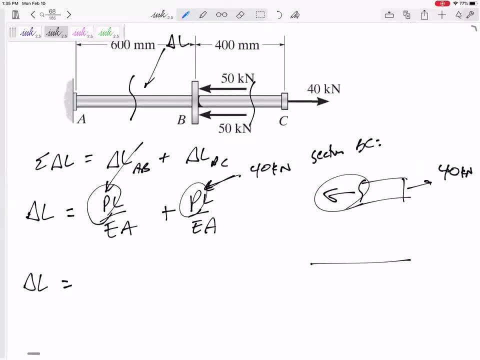 so i'm going to put in positive 40 right there. what about this force p inside this section? well, let me cut it all right. so i've got 40 kilonewtons there, but then i've got 50 and 50 right here. so summing: 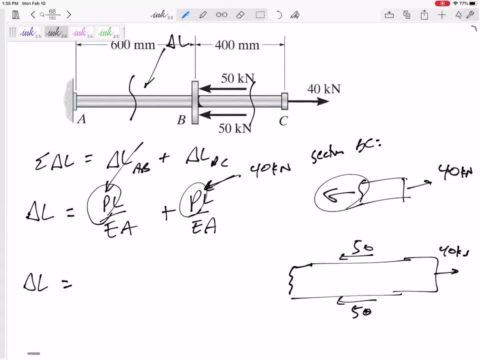 the forces in the x direction equals zero. uh, do you see that i would need 60 right there? i'm going to do 60 kilonewtons right there for that p, because it's 60 kilonewtons in compression. now i'm probably not going to do kilonewtons, i prefer newtons. 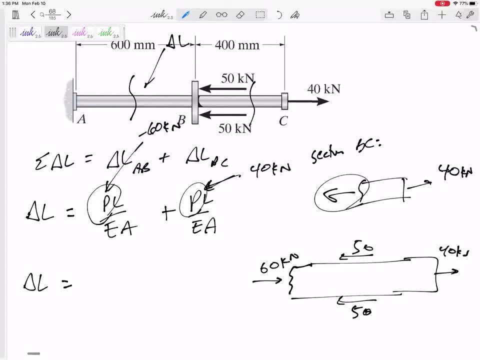 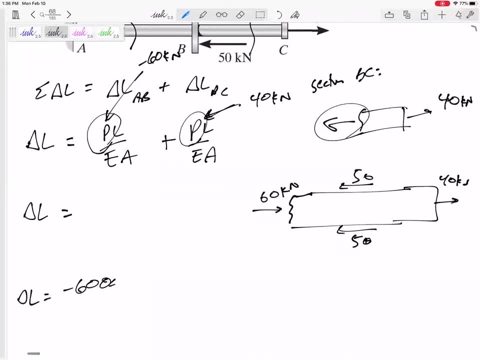 all right. so now the pl over ea. let me do some more room right here. all right, negative 60, i'm gonna do 60, 000 newtons the length of that section, 600 millimeters over the e 200. change it to 200, 000 so that i could do mpa and the area pi by 4, 20 squared. all right, so y'all. 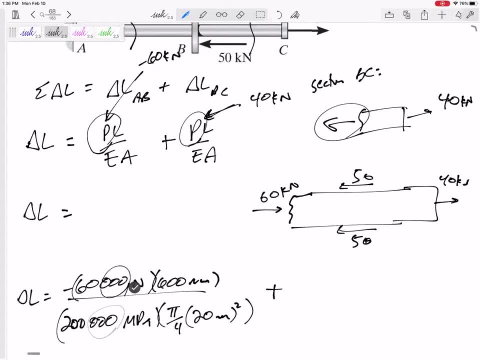 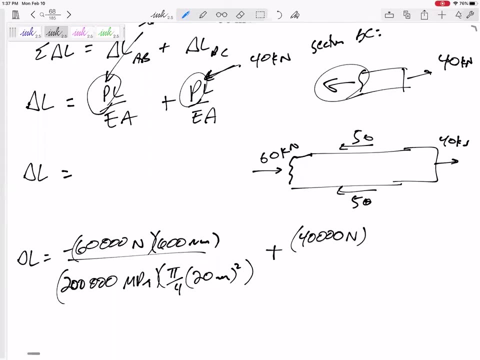 smarter than me, you know. maybe you just left kilonewtons and gpa. uh, those, those would be fine, but i prefer newtons, mpa and millimeters squared. all right, the next one: 40 000 newtons length is 400 millimeters over e, 200 000 mpa and pi by 4, 20 squared, and so there that will give me. 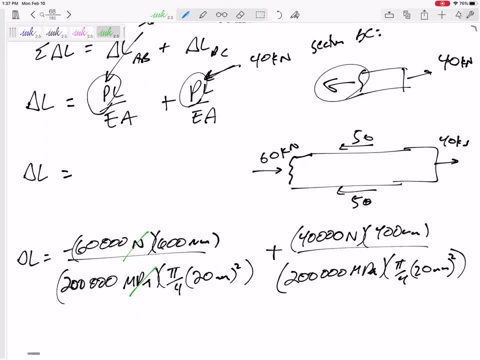 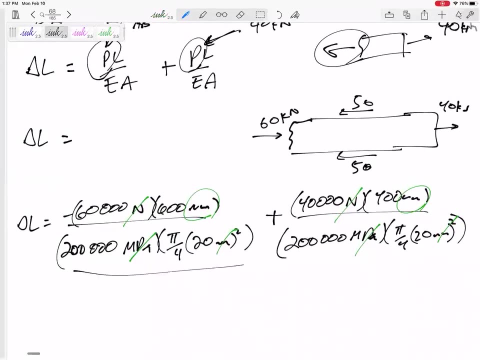 my delta l, the units newton, mpa and millimeter squared cancel out. so so yeah, my units for both of those terms are millimeters, so i could add them up. you probably could see that i could. i could have factored that out and only multiplied the e and the. 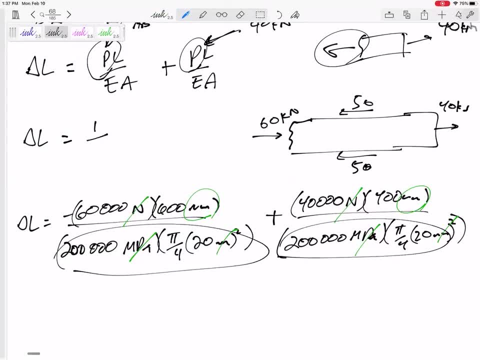 a once right. i could have said one over ea, pl plus pl right, things that are constant for every term you could cancel out. but it's a little bit more mad punching things into your calculator. but i just fall back to pl over ea of that section, pl over ea of that section. so